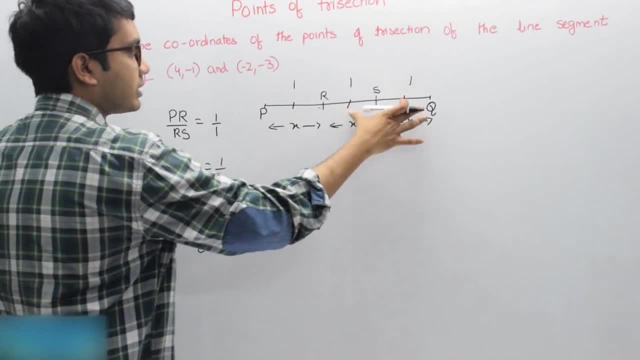 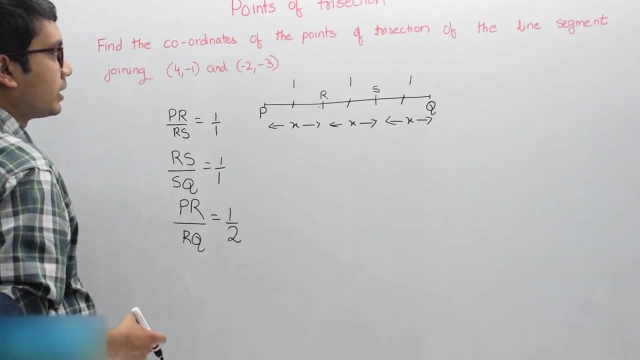 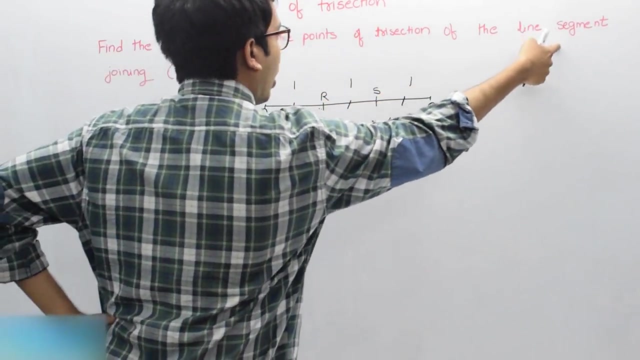 one by two because this is two parts. this is one part So I wrote it as PR by RQ is equal to one by two. Let us apply the concept here. So he says that find the coordinates of the points of trisection of the line segment joining. 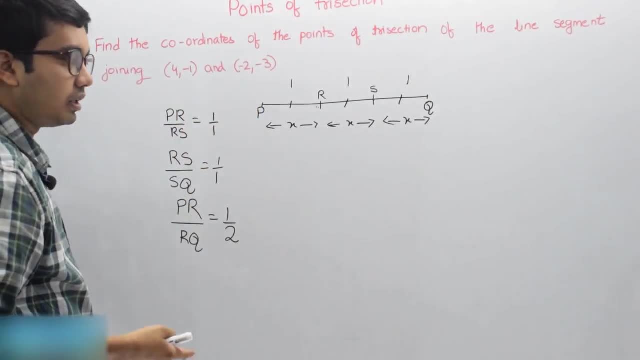 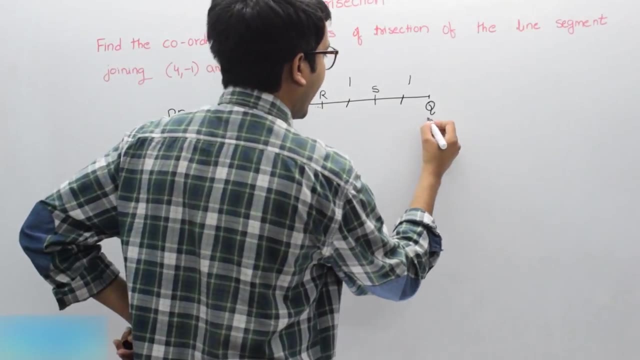 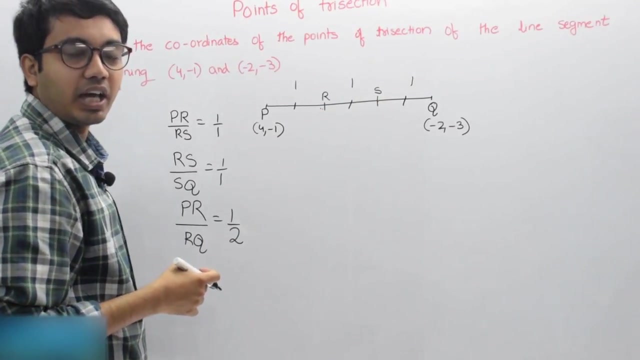 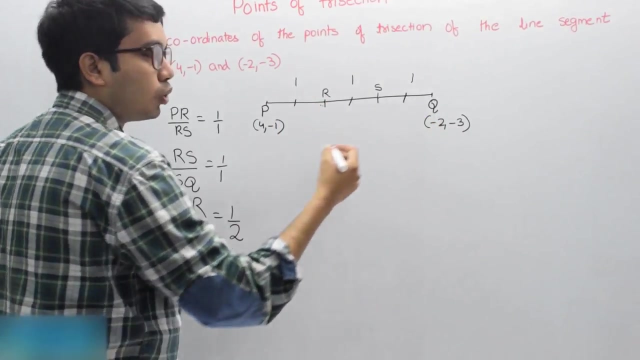 four comma minus one and minus two comma minus three. So let us assume this P as four comma minus one and Q as minus two comma minus three. I want the coordinates of R and S. We have learned about the internal division of line segment. Now R is dividing P and Q. 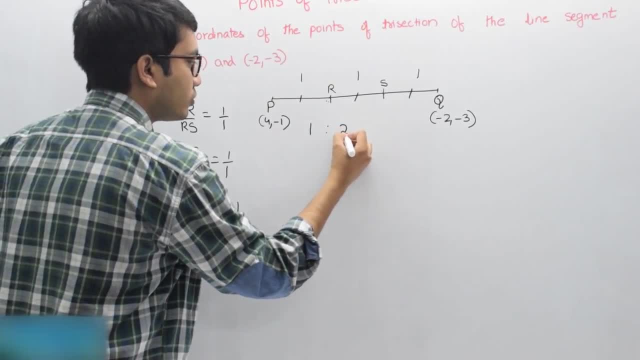 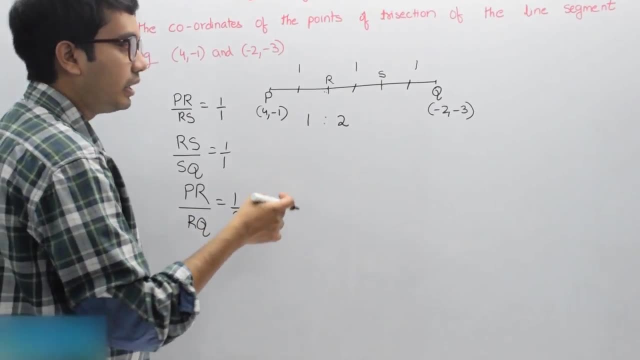 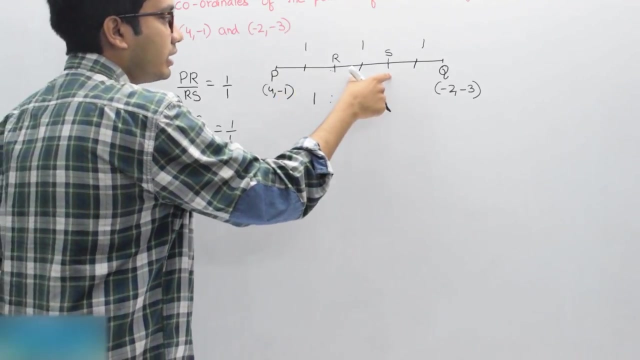 internally in the ratio one is to two, because previously I have told you that PR by RQ is equal to one by two. Simply R is dividing this line, segment PQ, in the ratio one is to two or this is one part, this is one plus one. 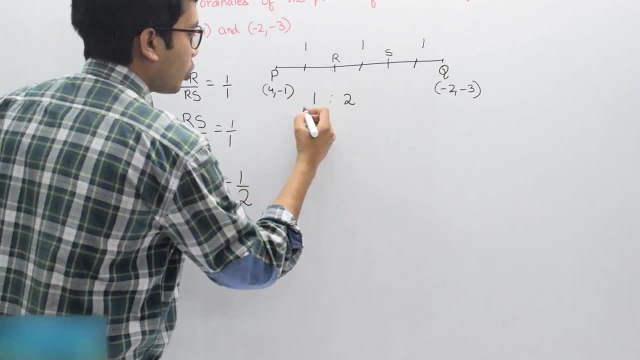 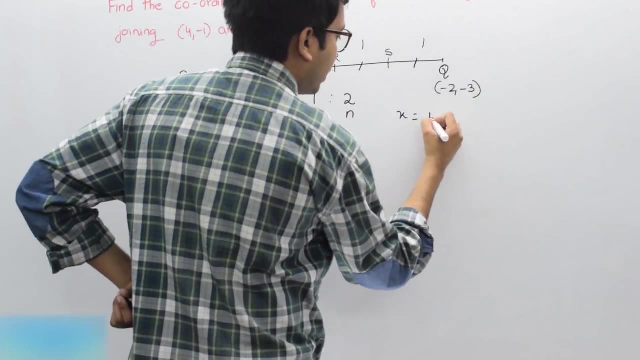 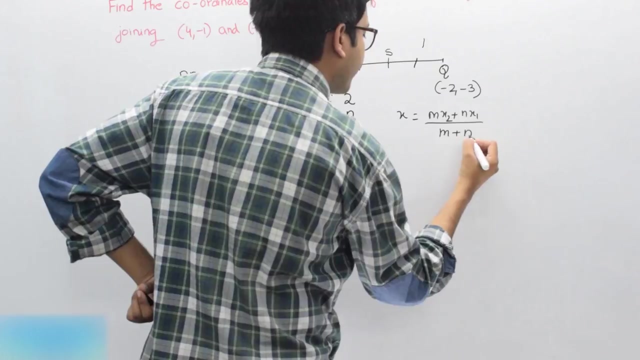 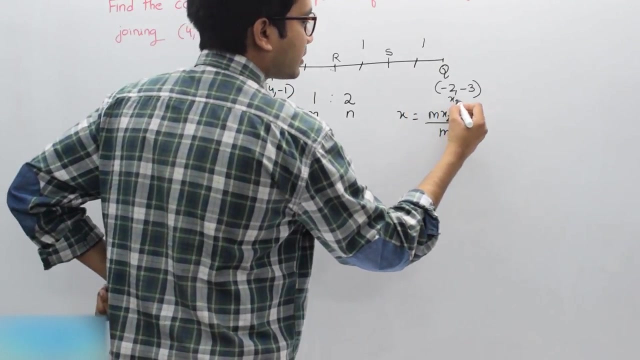 two parts. RQ is two parts, So here M will be one and N will be two. So applying X is equal to MX, two plus NX, one by M plus N. So I'll have this as X, one by one, point, P and Q as X, two, Y, two. I'll. 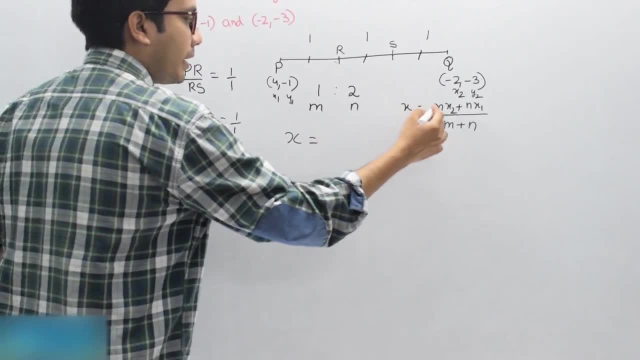 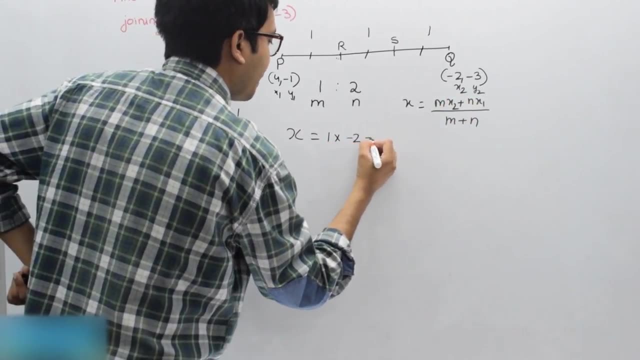 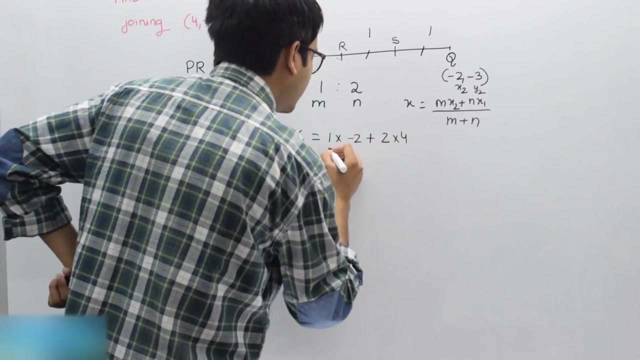 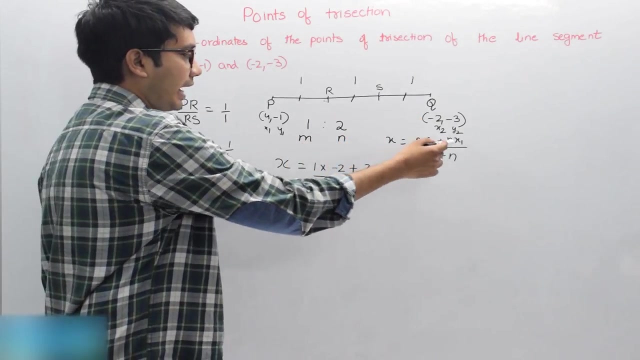 have X as MX two, that is, one into minus two plus NX one, two into four. So we have the X coordinate as MX two, that is one into minus 2 plus NX one, two into four by M plus N. Now let us see some other. 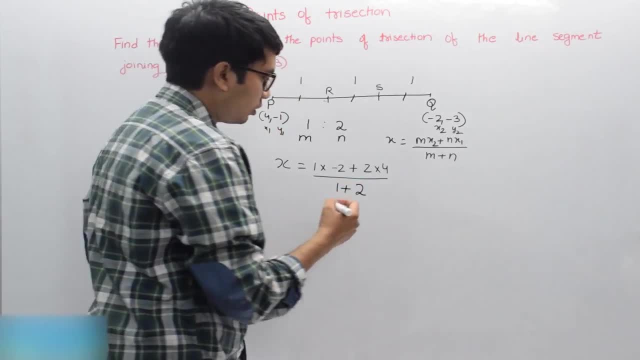 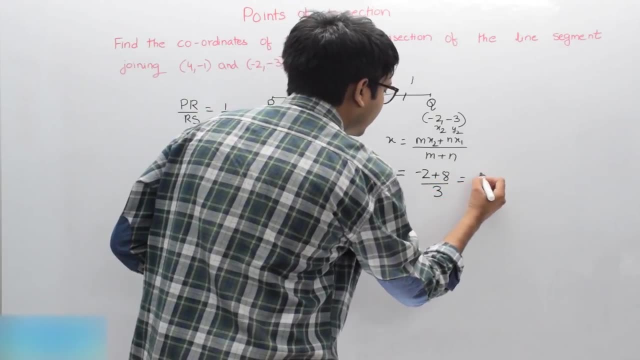 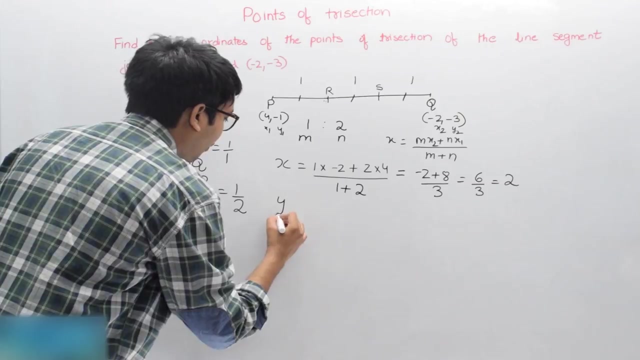 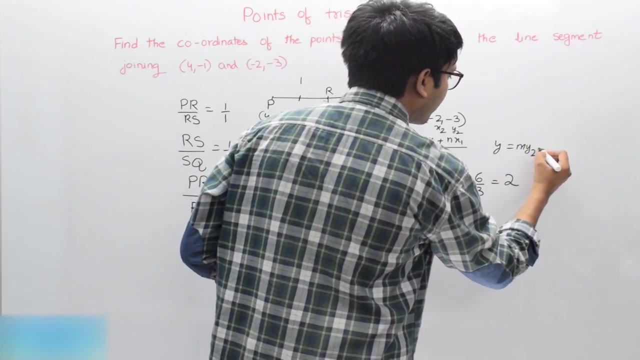 That is 1 plus 2.. So this is equal to minus 2 plus 8 by 3.. This is equal to 6 by 3, which is equal to 2.. Next we will have y, which is equal to m by 2 plus n, by 1 by m plus n. 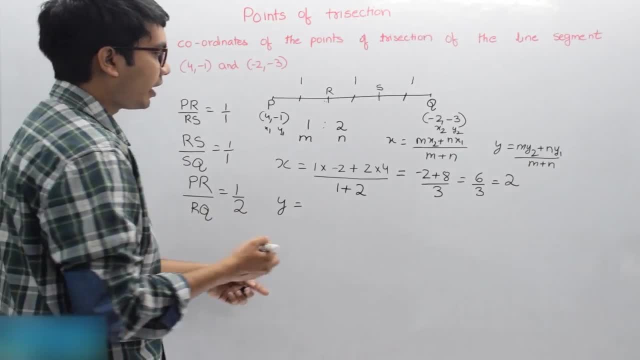 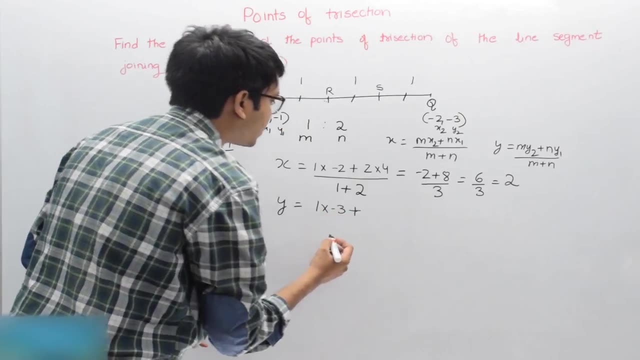 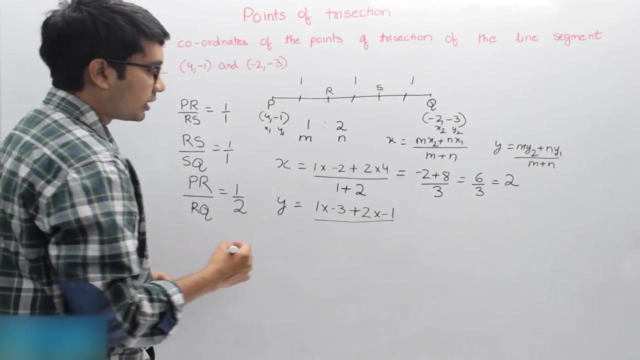 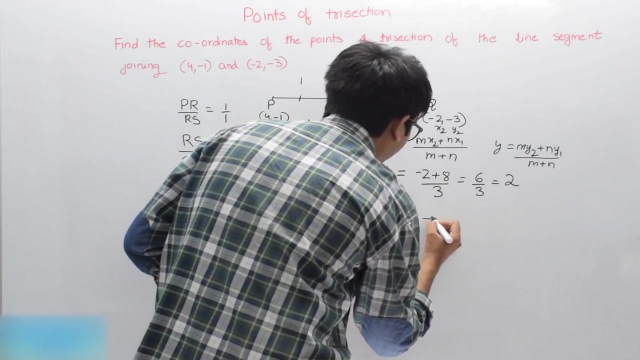 So that is: m by 2 is 1 into minus 3 plus n by 1,, 2 into minus 1 by m plus n, that is 1 plus 2.. So we have minus 3 minus 2 by 3, which is equal. 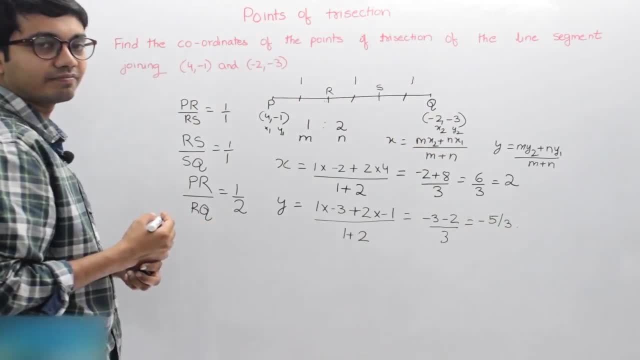 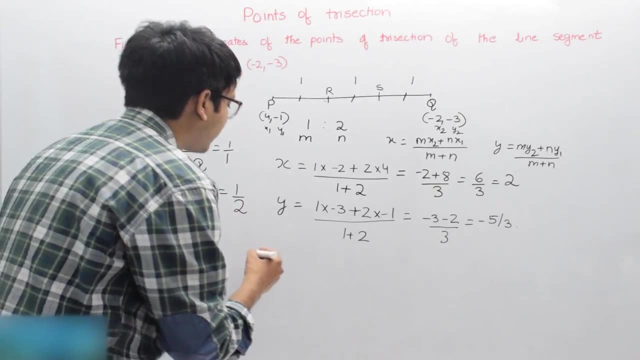 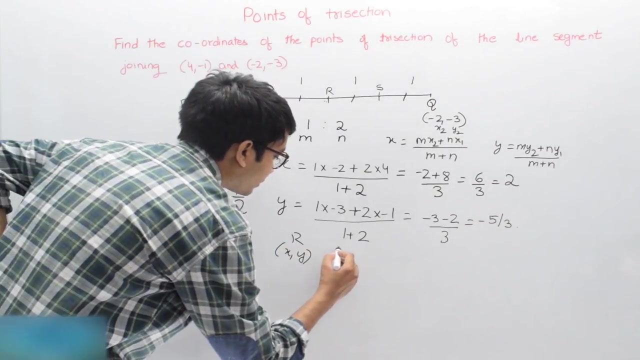 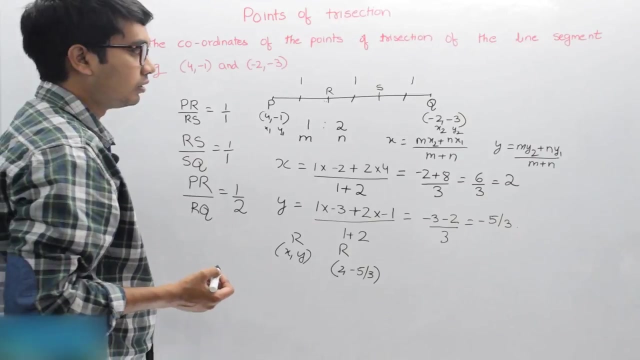 to minus 8. 5 by 3.. So what we did, We got x as 2 and y as minus 5 by 3.. So x comma y for R, that is, the coordinates are 2 comma minus 5 by 3.. So next let us try to find out the coordinates. 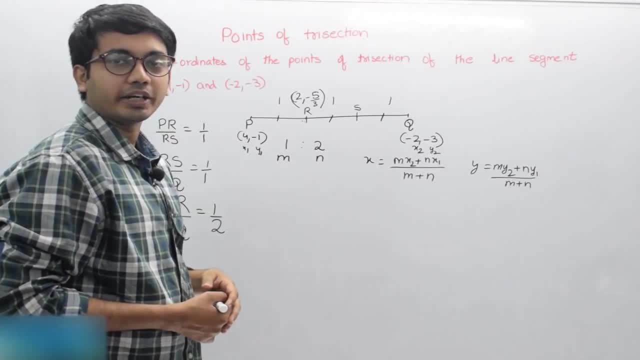 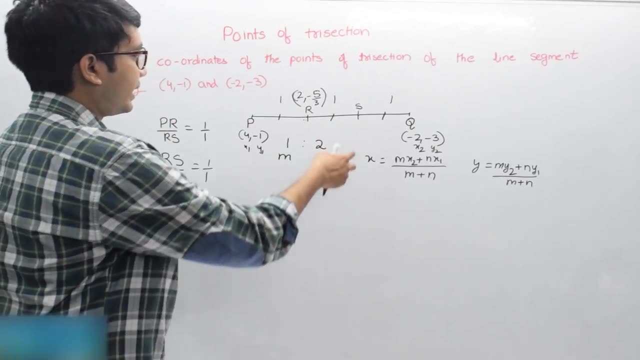 of S. We have got the coordinates of R. they are 2 comma minus 5 by 3, and let us try to find out the coordinates of S. This S divides P- Q. in the ratio 2 is to 1, because this is: 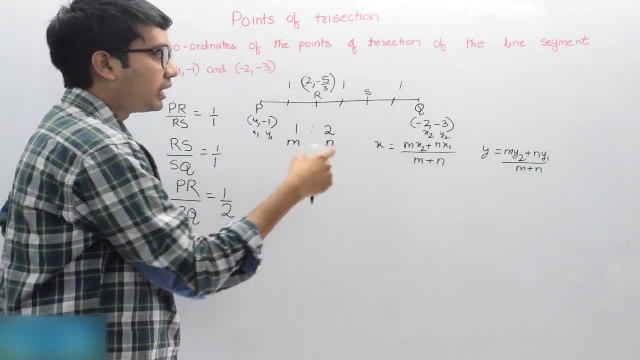 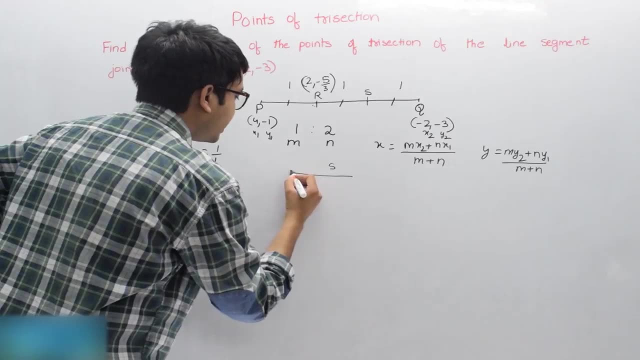 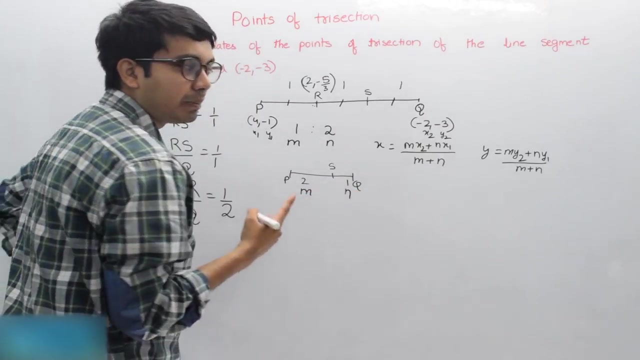 one part and this is one part. This total P S will be two parts and S- Q will be one part. So S divides this P and Q in the ratio of 2 is to 1.. So M will be 2 and N will be 1.. So this point, S is dividing P Q in the ratio. 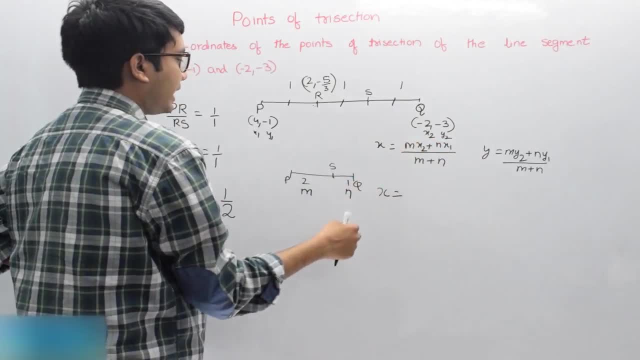 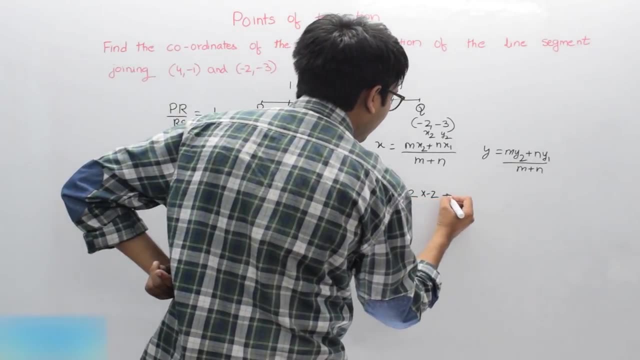 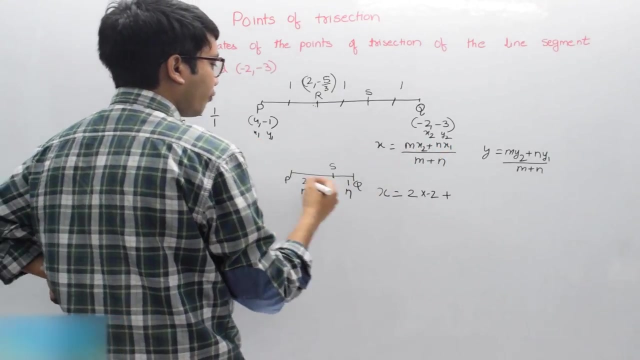 2 is to 1.. So our formula is M x 2 plus N x 1,, that is 2 into minus 2 plus N, that is 1 into he says x 1.. So it will be 4 by M plus N. 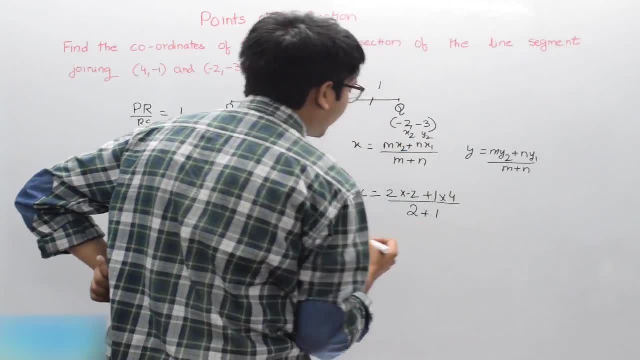 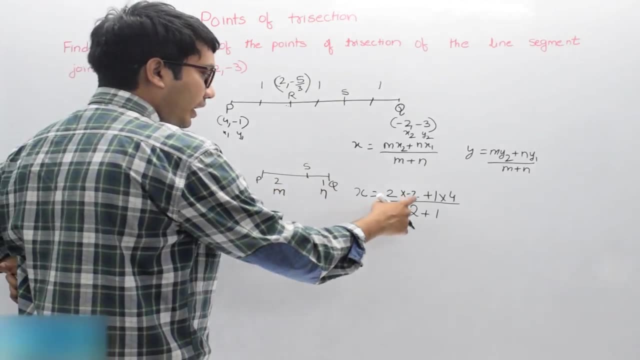 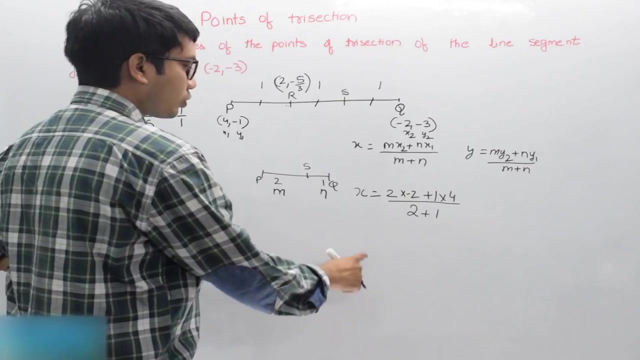 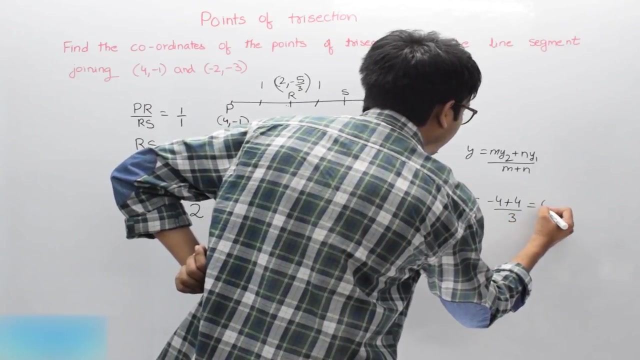 M plus N is 2 plus 1.. Listen, this S is dividing this line segment internally. that is why we are writing M plus N. If it divides externally, minus will come here and here. So this will be minus 4 plus 4 by 3, this is 0 actually We will have. y is equal to minus 4 by 3.. So 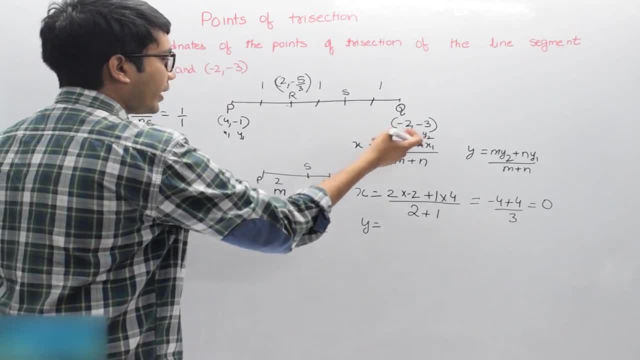 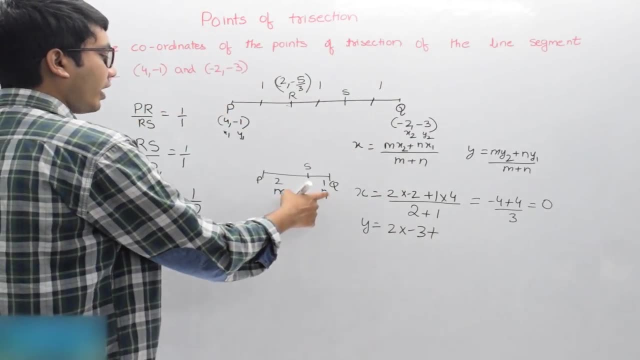 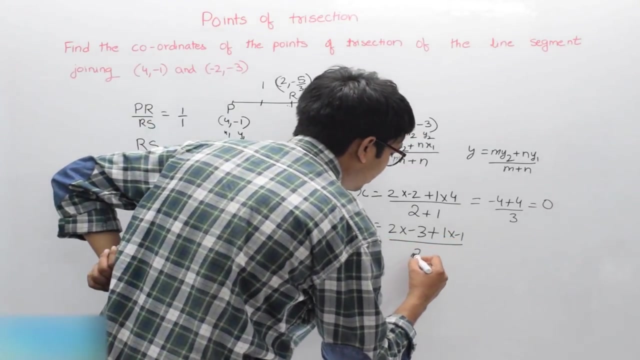 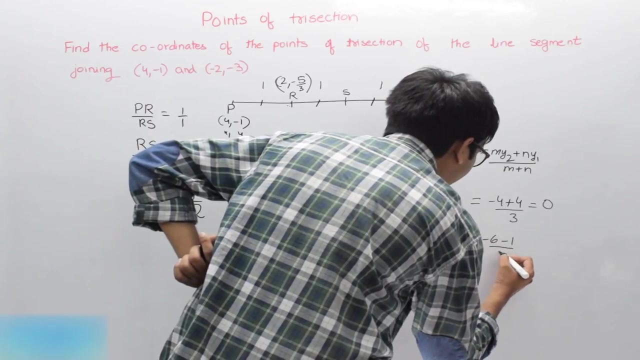 M y 2 plus N y 1 by M plus N 2 into y 2 minus 3 plus N y 1, 1 into minus 1 by M plus N 2 plus 1. This will be equal to minus 6 minus 1 by 3.. current. square, So which is equal to minus 7, plus 1.. Merger 4 plus automatically multiply. we chose the current. now V will replace the P Q in the relation and you can take this into・M by M plus N, So that will be M x 1 de. 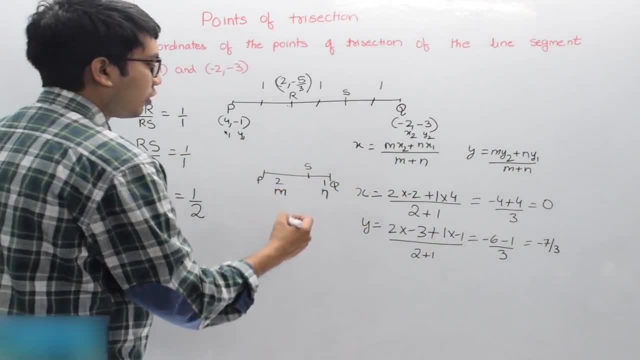 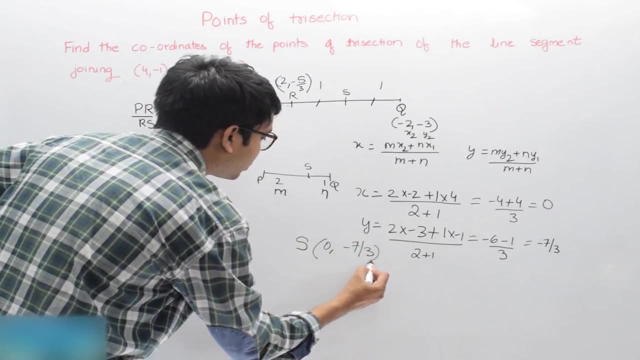 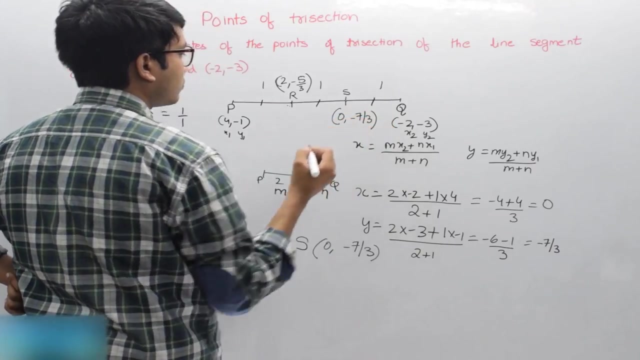 which is minus 4 plus 4 by 2 plus 1.. So we have x 2 plus 2 plus 1 into minus 3, this will be 3.. So we have the coordinates of S as 0 comma minus 7 by 3. So the coordinates of R are: 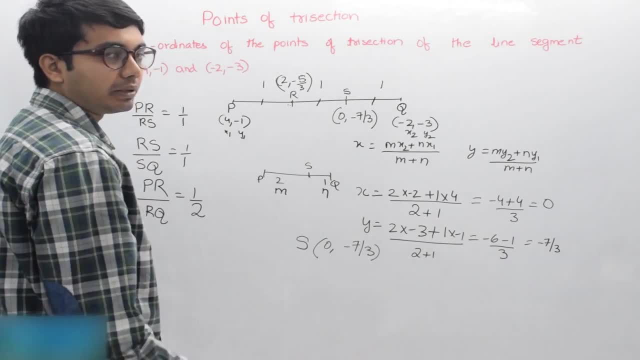 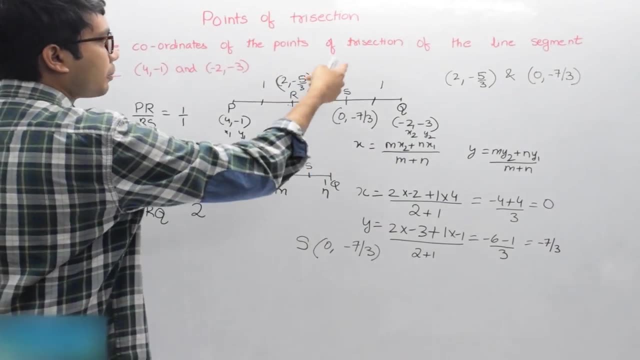 2 comma minus 5 by 3 and S are 0 comma minus 7 by 3.. So I can say 2 comma minus 5 by 3 and 0 comma minus 7 by 3 are the points of trisection of the line segment joining these. 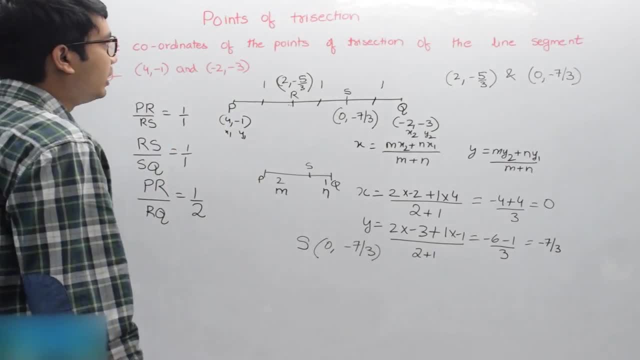 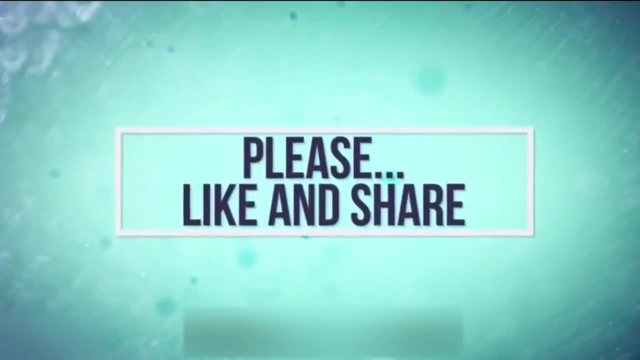 two points, that is, 4 and minus 1 and minus 2 and minus 3.. This is the concept of points of trisection. Thank you. If you like the video, please hit the like button, comment and share it with your friends. Also, don't forget to subscribe for all our future videos. 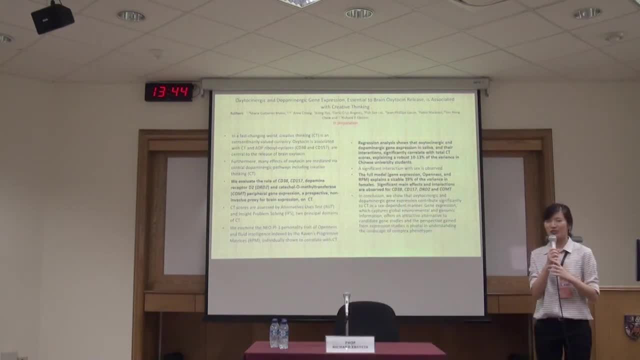 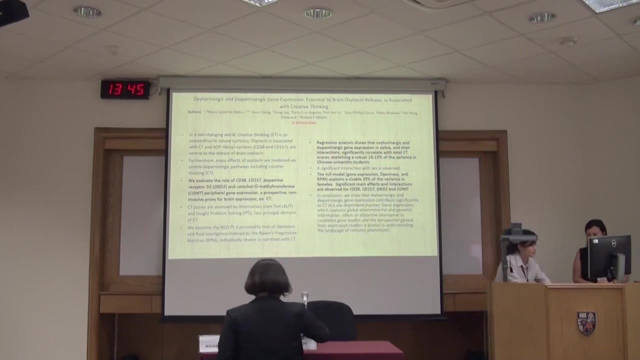 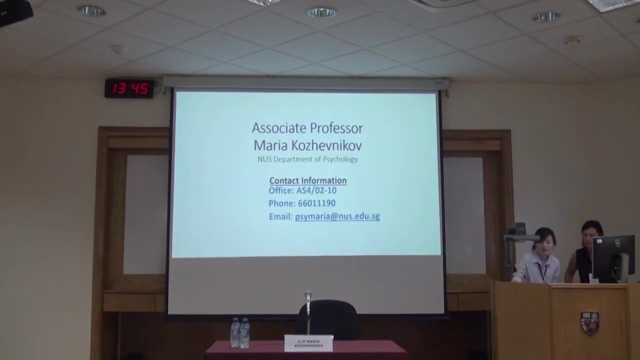 This is a non-atomic speaker by Professor Maria Kuczyn-Pikul. Okay, so I will talk about individual differences in optic versus spatial visualization, And this is a brief outline. I start with the ground and then I'll show a few of my studies on this topic.